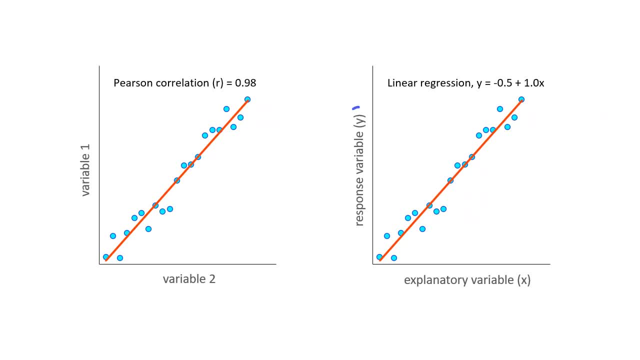 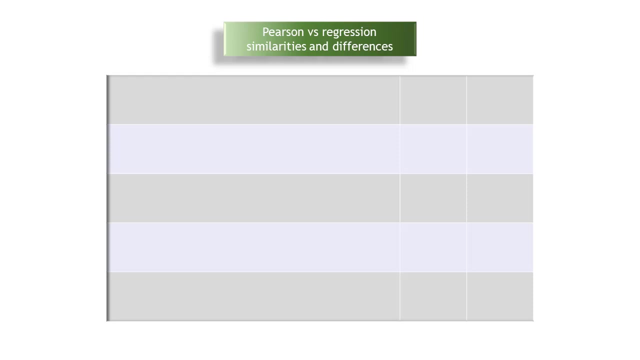 Linear Regression describes the linear relationship between a response variable denoted by y and an explanatory variable denoted by x, using a statistical model, and this model can be used to make predictions. Let's examine the key similarities and differences between Pearson Correlation and Simple Linear Regression. Both can be used to quantify the direction. 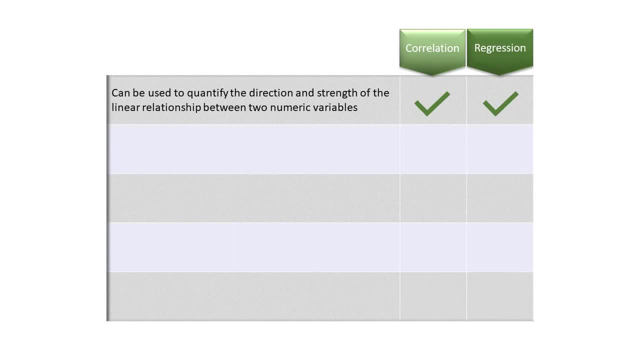 and strength of the linear relationship between two numeric variables. However, only regression predicts how the explanatory variable x causes the response variable y to change With correlation. both variables are assumed to be random, whereas for regression, only the response variable y is assumed to be a random variable. The explanatory variable x is assumed to be fixed. 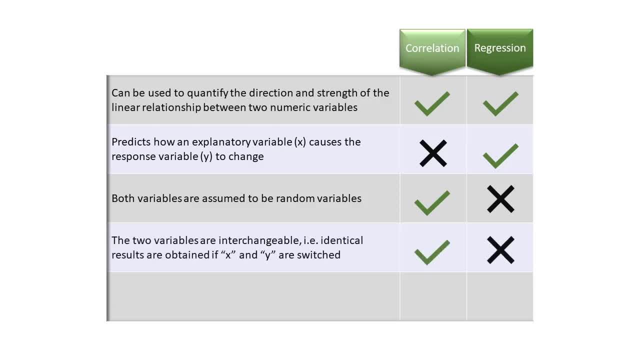 and measured without error. When calculating a correlation, you can swap the two variables around without affecting the results. However, for regression, if you interchange the explanatory and response variables, the results will also change. Finally, regression produces a statistical model, whereas correlation is a simple descriptive statistic. 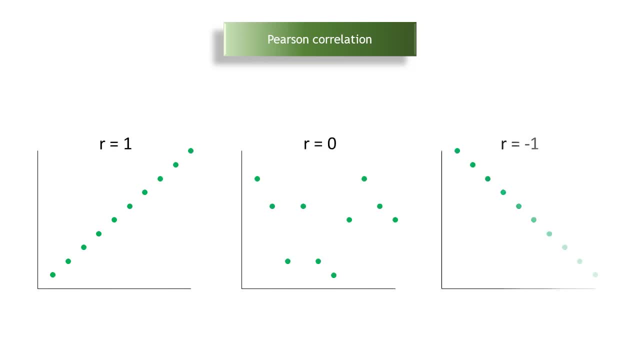 Let's look at Pearson Correlation in more detail. Pearson Correlation is a number ranging from negative 1 to 1 that represents the strength of the linear relationship between two numeric variables. The Pearson Correlation is also known as the Product Moment Correlation Coefficient or simply Correlation. 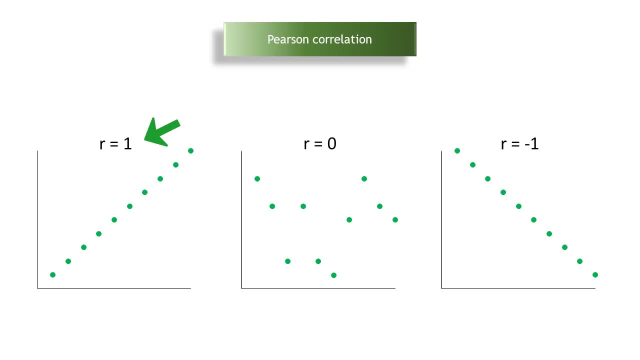 A value of 1 corresponds to a perfect positive linear relationship, A value of 0 means there is no linear relationship and a value of negative 1 is a perfect negative relationship. The Pearson Correlation denoted by R between variables x and y is calculated with the help. 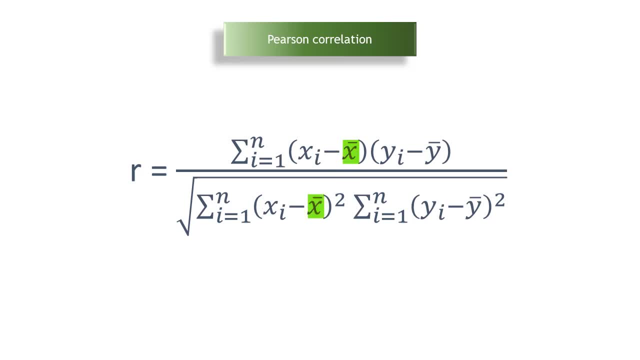 of this formula. Here, x-bar is the mean of the x-values and y-bar is the mean of the y-values. The character n represents the sample size. Later on we'll show you how to calculate the Pearson Correlation using GenStat. 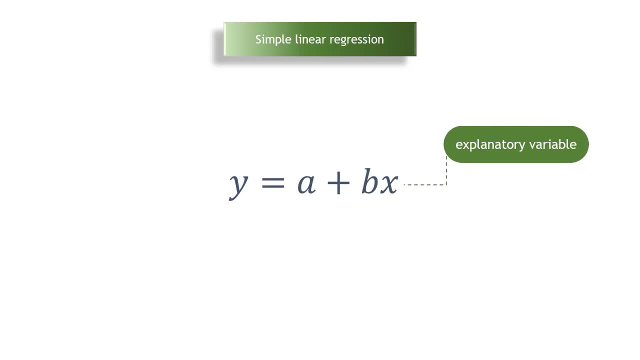 When we're interested in the effect of an explanatory x variable on a response y variable, a regression analysis is appropriate. A regression describes the response variable y using this model. Here the coefficients a and b are the intercept and slope of the regression line. The intercept a is the value. 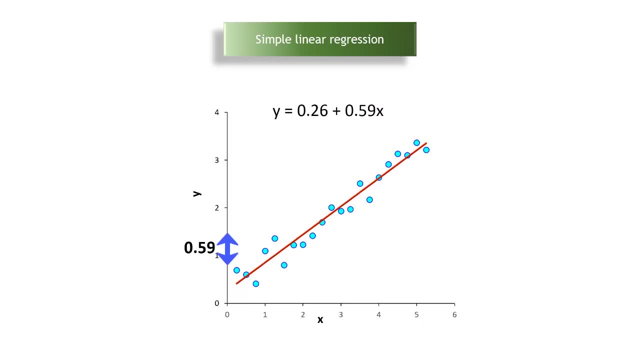 of y when x is 0. The slope b is the change in y for every 1-unit increase in x. When the correlation is positive, the slope of the regression line will also be positive, and vice versa. The model is theoretical. 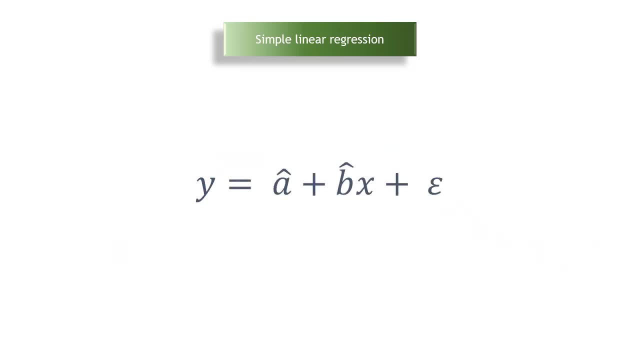 And in practice there will be error. The statistical model is given by this formula, where epsilon, a barrier of residuals, represents the difference between the predicted y-values and the observed y-values. The hat accent is used to denote values estimated from the observed data, The regression coefficients. 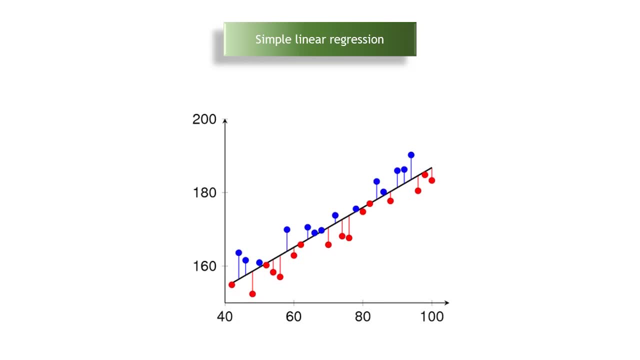 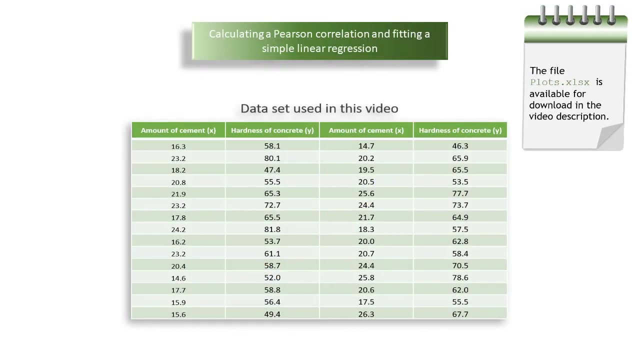 a and b are estimated by least squares. This results in a regression line that minimizes the sum of the squared residuals. Let's now demonstrate how to calculate a Pearson correlation and fit a simple linear regression in GenStat. The example we'll use is from a concrete manufacturer who wants to know if the hardness of their 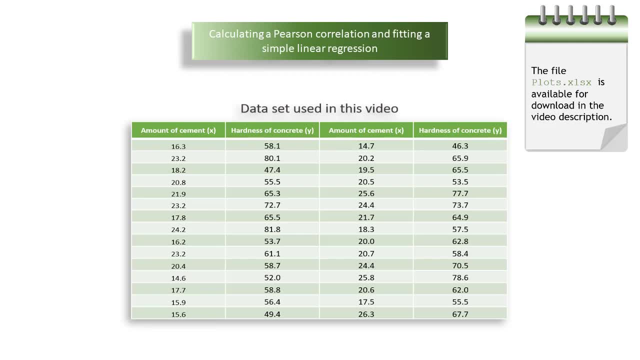 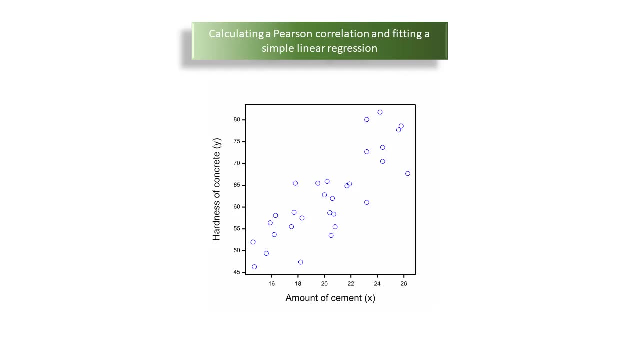 concrete depends on the amount of cement used to make it. They collected data from 30 batches of concrete. The scatter plot of the data suggests that the two variables are linearly related. Let's first assess whether there is evidence of a significant correlation between the two variables. 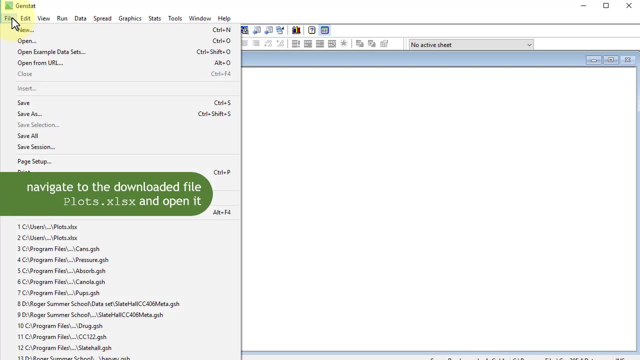 Let's first assess whether there is evidence of a significant correlation between the two variables. Let's first assess whether there is evidence of a significant correlation between the two variables. We will test for evidence of a significant Pearson correlation between the hardness of the concrete and the amount of cement used to make it. Our null hypothesis is that true. 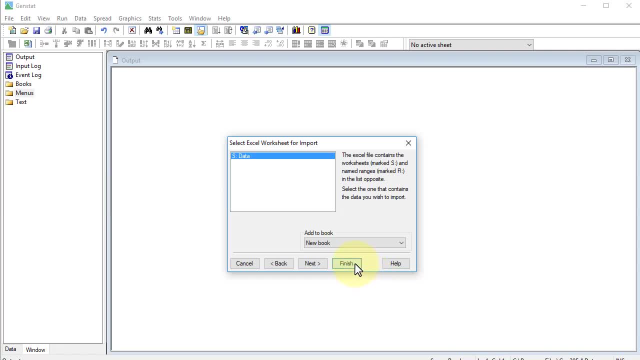 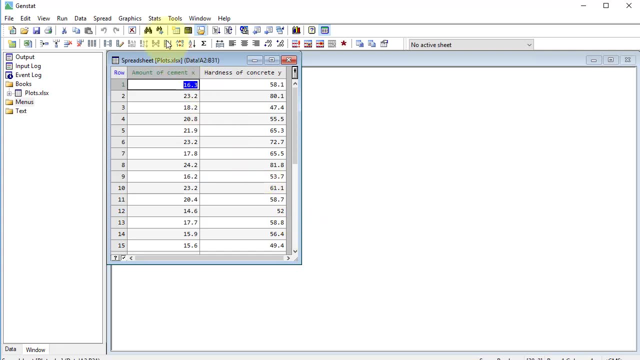 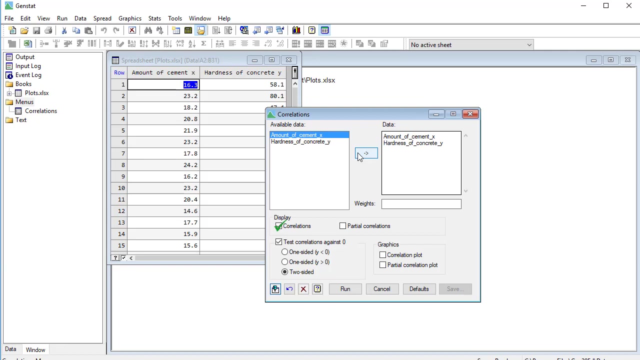 correlation equals 0.. Using GenStat, we can calculate the Pearson correlation and test for evidence against our null hypothesis. using the correlations menu. Select stats- summary statistics- correlations- Select the two variables that we want to correlate. Now select Correlations as the output to display. 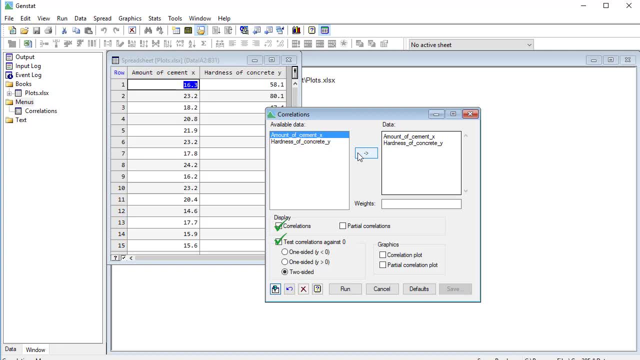 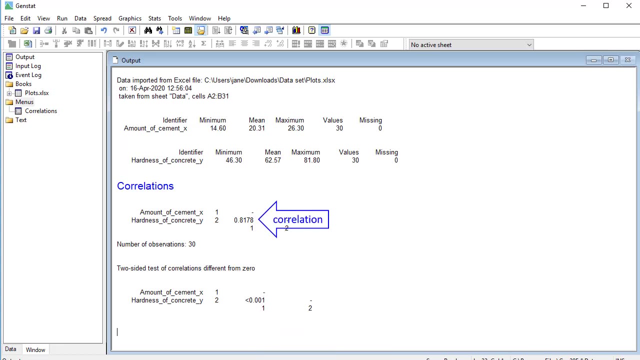 We also want to test the null hypothesis, that true correlation equals zero, against the two-sided alternative hypothesis that the true correlation is not equal to zero. Click, Run and let's see the output. We can see that the correlation estimated from the data is 0.82, with a p-value of less. 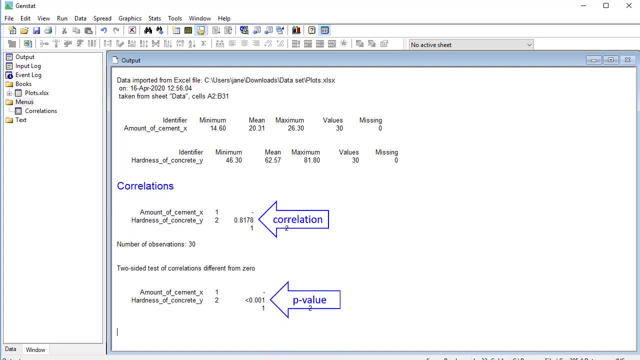 than 0.001.. That is, there is strong statistical evidence of a linear relationship between the two variables. The validity of our hypothesis test depends on several assumptions, including that x and y are continuous, jointly normally distributed random variables. If the scatter plot indicates a non-linear relationship between x and y, the bivariate 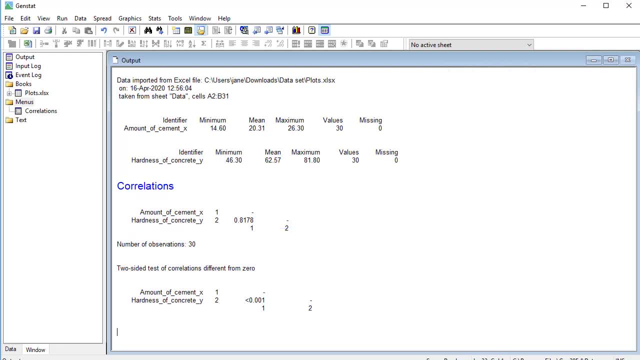 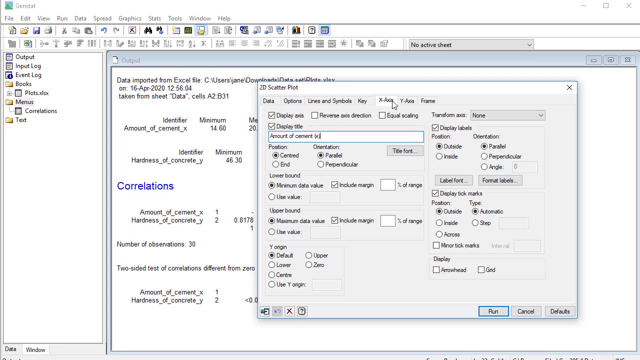 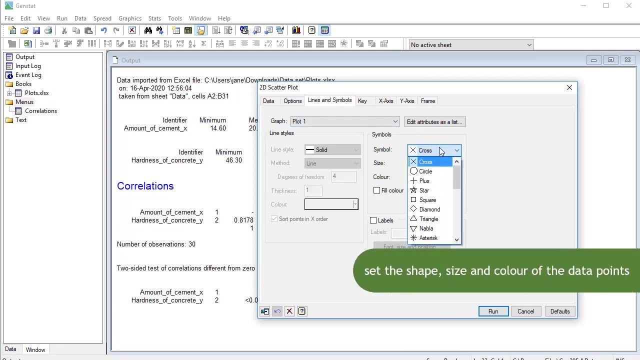 normal assumption is violated. Let's recreate the scatter plot that you saw earlier in this video. We select Graphics 2D Scatter Plot And I'll fill in the forms quickly to show you how it's done. You can always pause the video if you need more time to take this in. 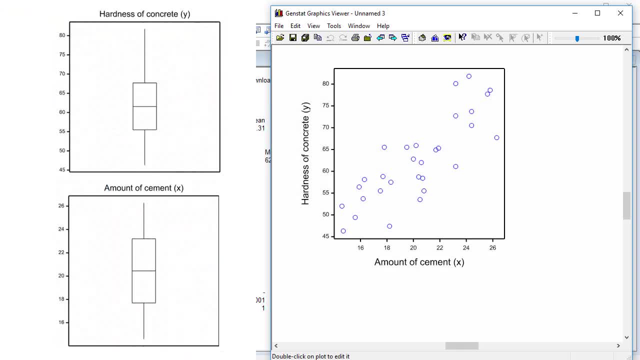 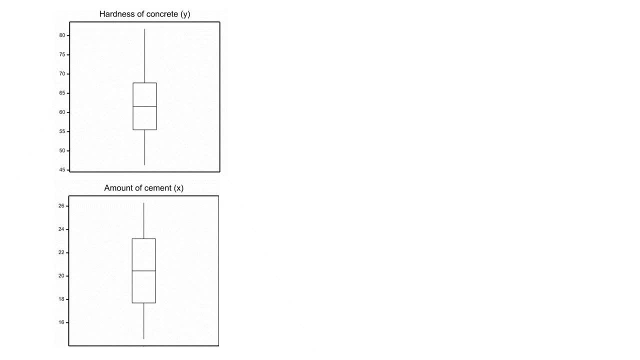 We can see that the scatter plot looks reasonably linear. We should also check that the scatter plot is linear. We can also check whether both the x and y variables appear to be normally distributed. This can be done graphically by inspecting, for example, a box plot, a histogram or qq. 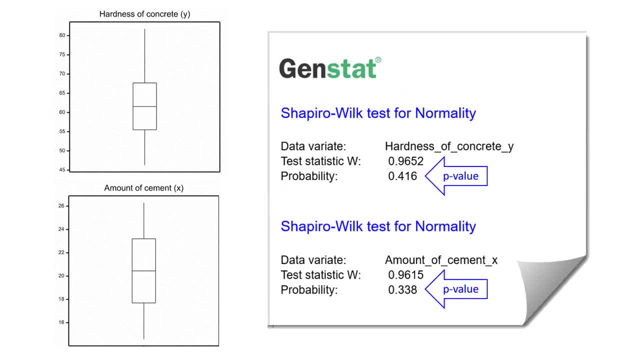 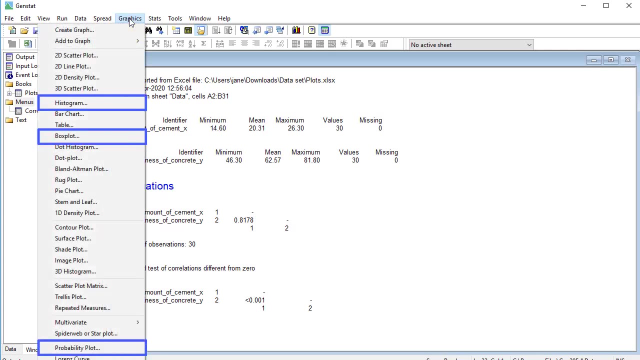 plot. Alternatively, we could perform a hypothesis test of normality, such as the Shapiro-Wilk test, For both variables in our dataset. neither their box plot nor Shapiro-Wilk test indicate a lack of normality. You can create plots using the Graphics menu. 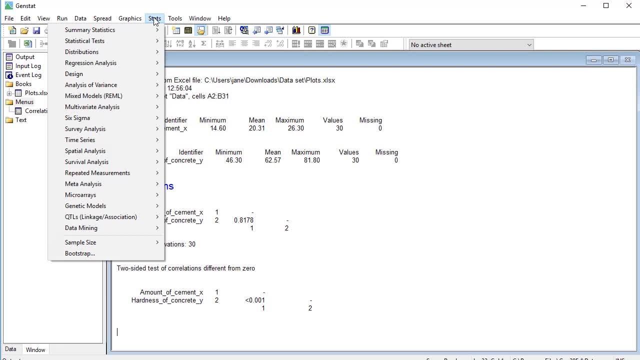 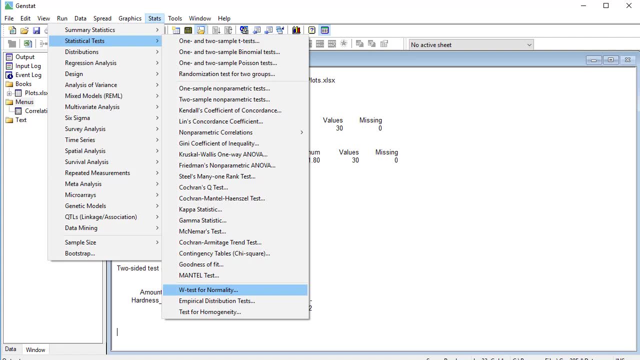 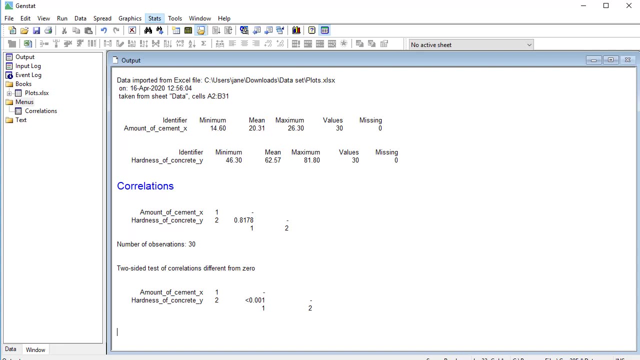 3D Scatter Plot. You can find the Shapiro-Wilk test by selecting Stats, Statistical Tests, W-Test for Normality. Going back to our dataset, as the hardness of the concrete is assumed to represent a response to changes in the amount of cement, it is more informative to model the data using. 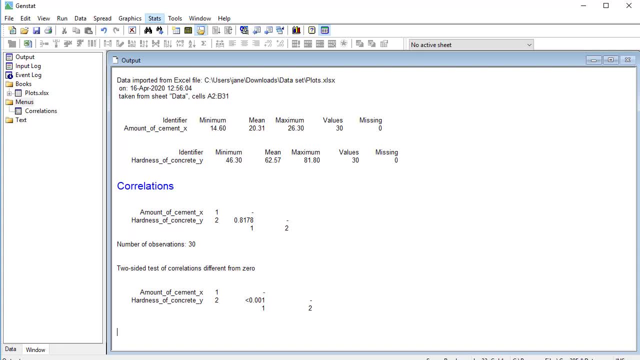 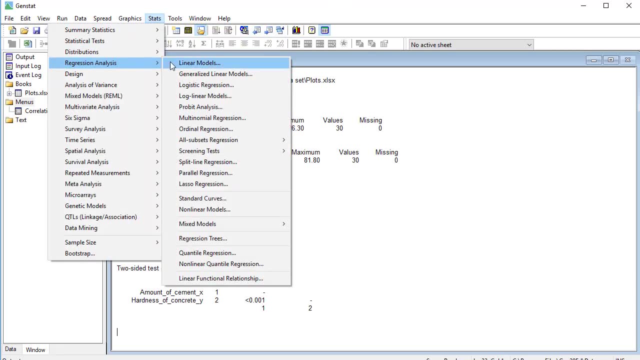 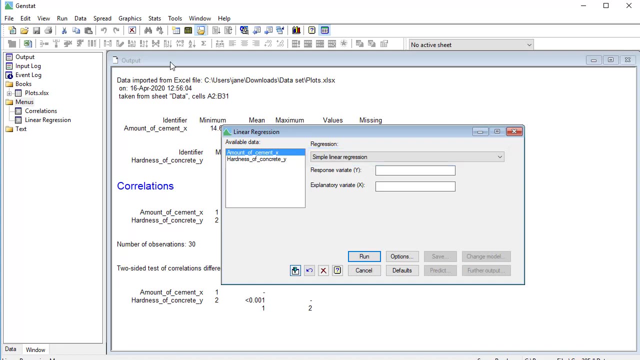 a simple linear regression. Let's open the Linear Regression menu and fit a simple linear regression. Select Stats, Regression Analysis, Linear Models. Then select Simple Linear Regression Recall. we want to see how concrete hardness responds to changes in cement amounts. Therefore, our response variable is the hardness of concrete. 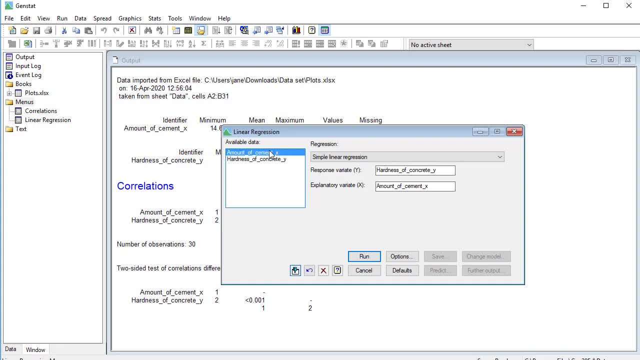 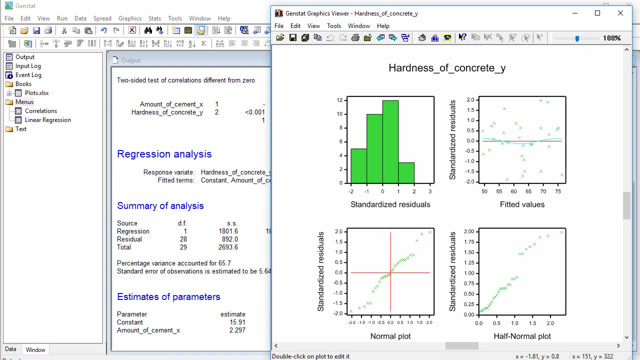 Our explanatory variable is the amount of cement. We'll open the Options menu to specify the output we want to see. Set these options, Click OK. Then click Run to fit the model. Before we examine the regression model, let's inspect the residual diagnostic plots to see. 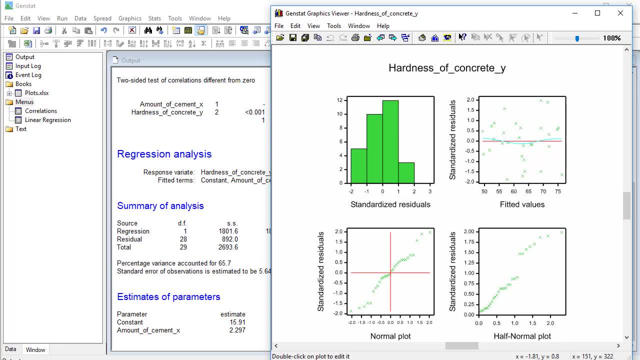 if the model assumptions appear to be OK, The residuals epsilon from the regression model are assumed to be independent and normally distributed with constant variance. The residual diagnostic plot is useful for helping check these assumptions. The histogram normal plot and half-normal plot are used to assess normality. 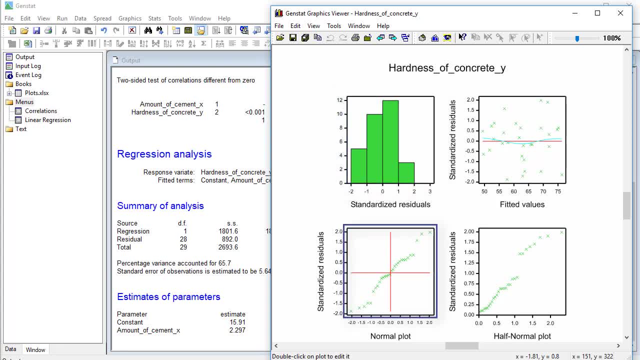 The histogram should be reasonably symmetric and balanced. The histogram should be reasonably symmetric and balanced. The histogram should be reasonably symmetric and balanced. Both the normal plot and half-normal plot should form roughly a straight line. The scatter plot of residuals against fitted values is used to assess the constant variance assumption. 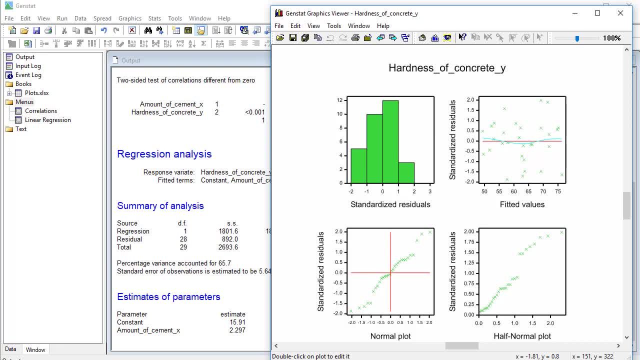 The spread of the residuals should be equal over the range of fitted values. It can also reveal violations of the independence assumption or a lack of fit. The points should be randomly scattered without any pattern. For our model, the residual diagnostic plot is used to assess the constant variance assumption. 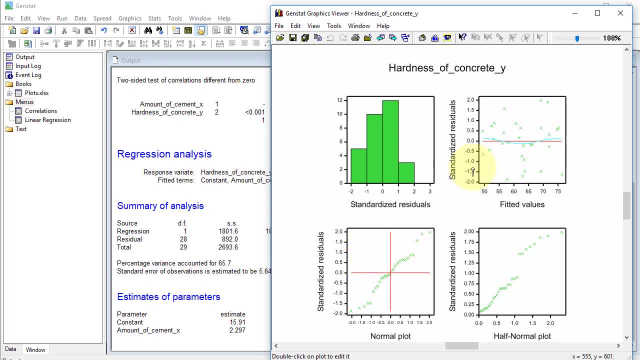 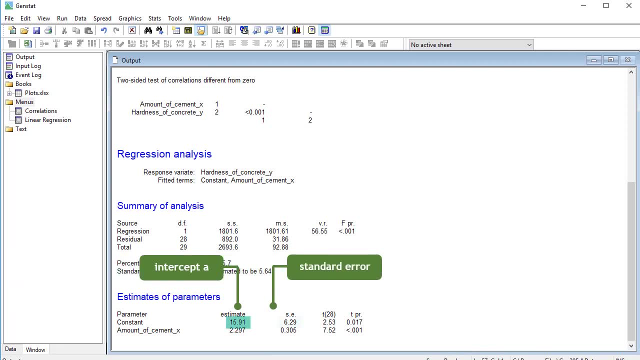 The spread of the residuals should be equal over the range of fitted values. It can also reveal violations of the independence assumption. Our report is to see that the possible results with inaccessible GC- 이것도見て, you may be creditable. however, this may not be the case for all models. 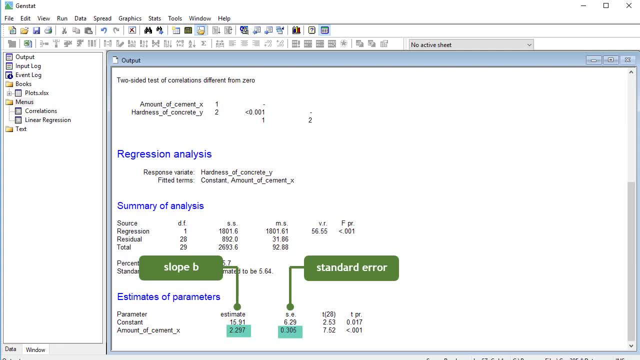 It may happen that the result is antenna as linear regression, but there is no benefit to units. We can write the equation for the regression line as follows For a simple linear regression: we're also interested in whether there is evidence of a linear relationship with the explanatory variable. 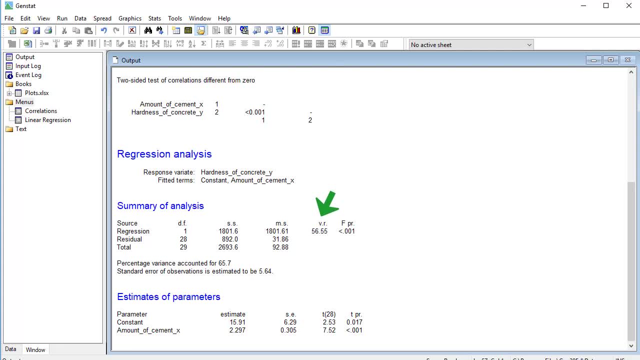 This can be assessed using the variance ratio, which, under the null hypothesis of no linear relationship, has an F-distribution. The p-value from this test is less than 0.001, providing strong statistical evidence of a relationship. The percentage variance accounted for summarizes how much variability in the data is explained. 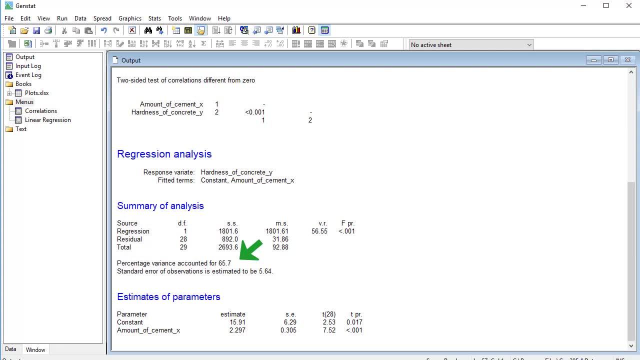 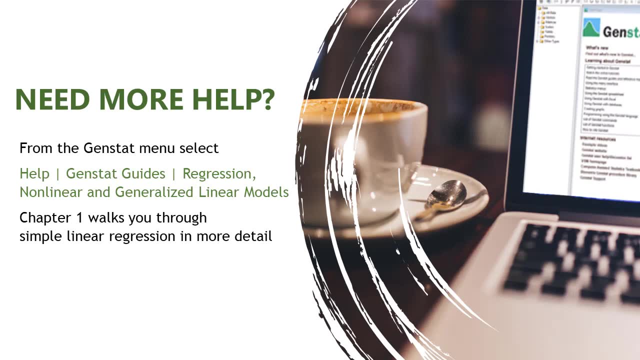 by the regression model in this example: 65.7%. Thank you. 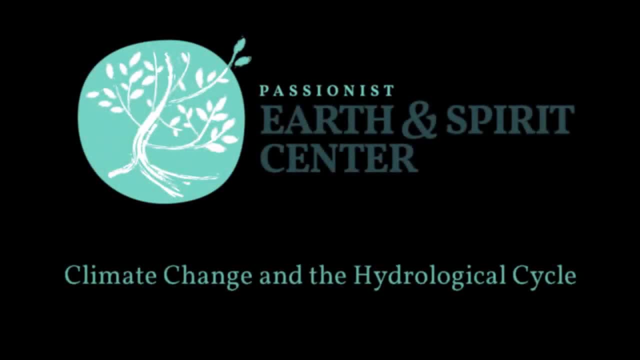 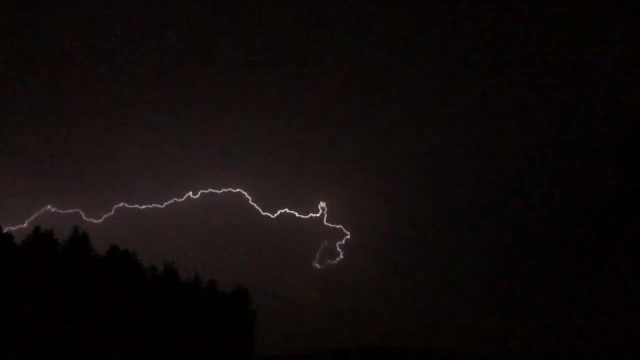 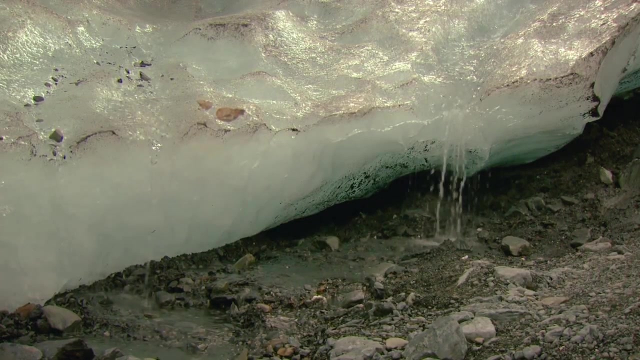 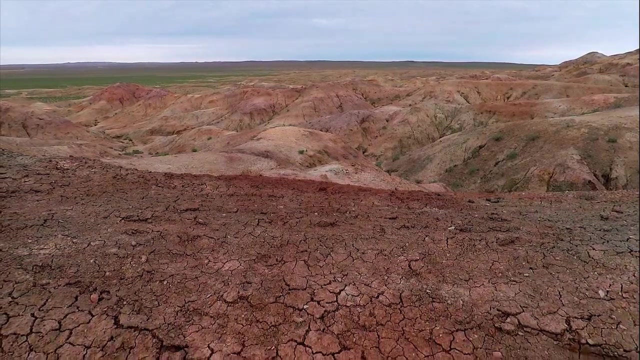 I don't know if you've noticed or not, but strange things have been going on with the weather lately. We've been having more rain and more flooding. The glaciers are melting at a faster rate and breaking off into the ocean. There have also been more droughts, where waterways are drying up and crops are. 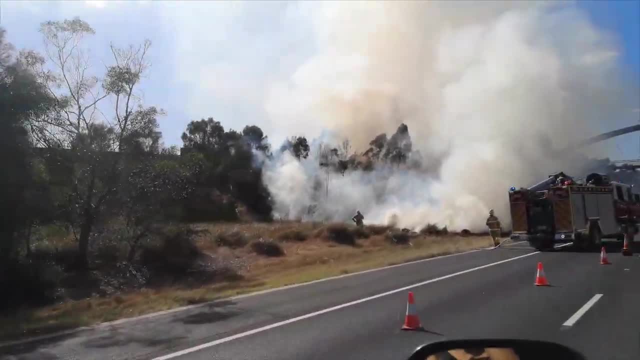 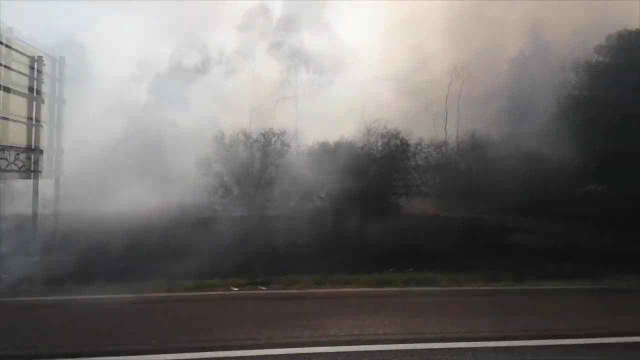 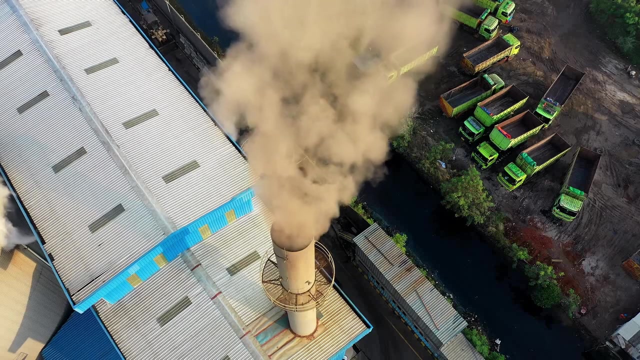 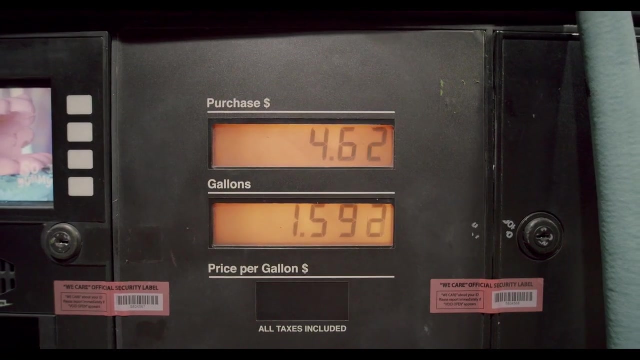 dying. A record number of forest fires have broken out around the world. What is going on? Well, the problem, you see, is that we're burning fossil fuels at an alarming rate, and the pollution from those fuels is causing the climate to change. We're also destroying our forests faster than they can grow back. This 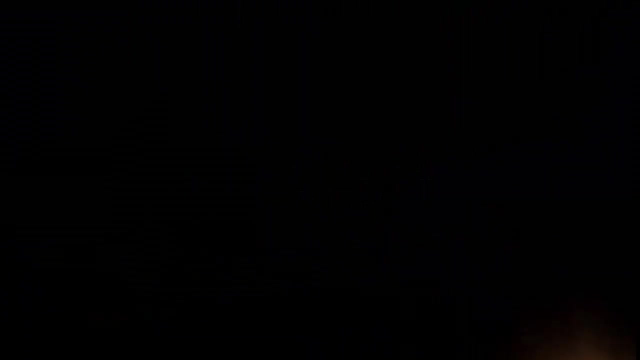 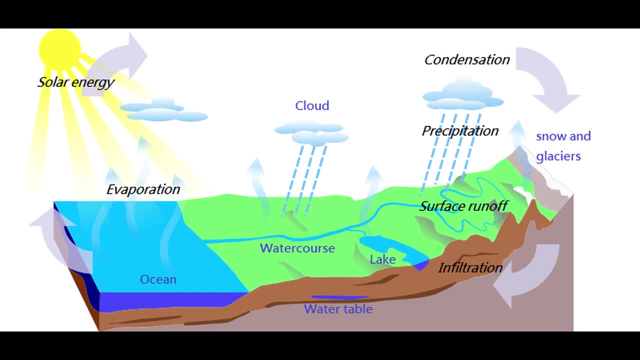 means that the planet is heating up and that it's wreaking havoc on our climate. To get a better understanding of this, we need to go back to our water cycle. Remember that The hydrological cycle gets its energy from the Sun, The heat. 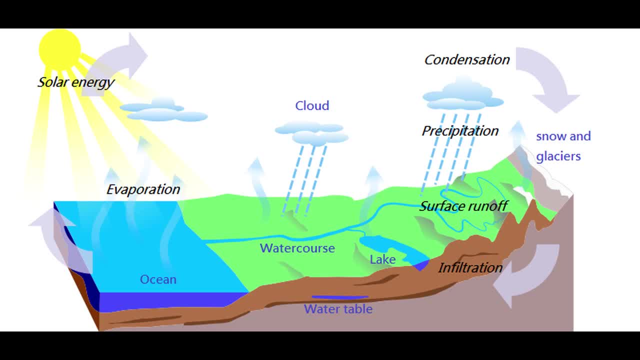 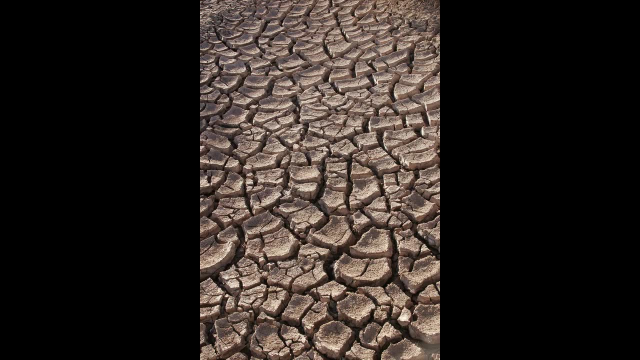 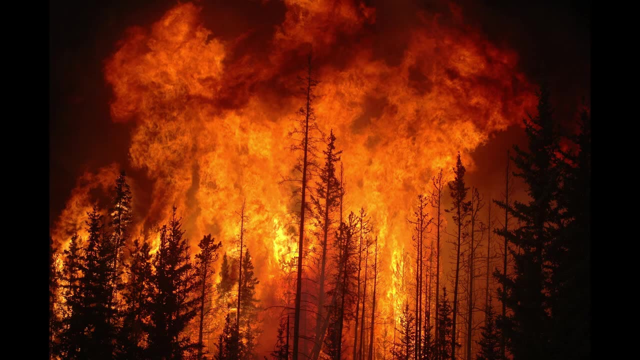 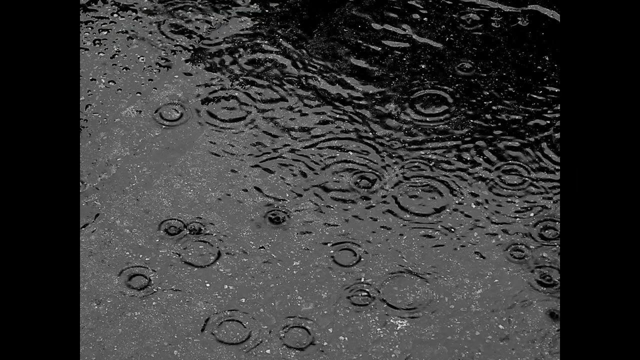 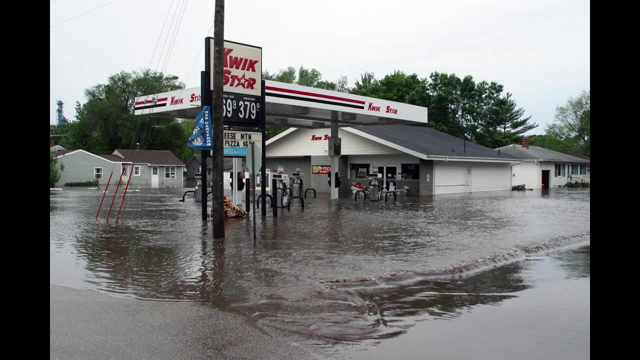 from the Sun causes evaporation and transpiration. A warmer planet means more evaporation and transpiration, So we have more droughts and forest fires and our waterways are drying up. It also means there is more water in the atmosphere, And what goes up must come down, So we are also seeing stronger storms more.